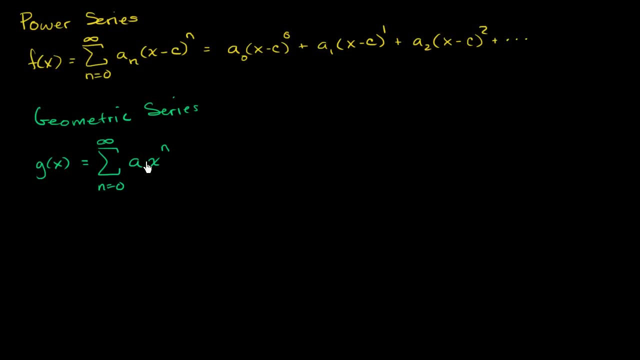 So this is kind of other words, sort of a Buttom Thing: pause for a second, pause for a second. This is kind of a typical geometric series here. And what's the difference between this and this? Well, the difference is here for every term. 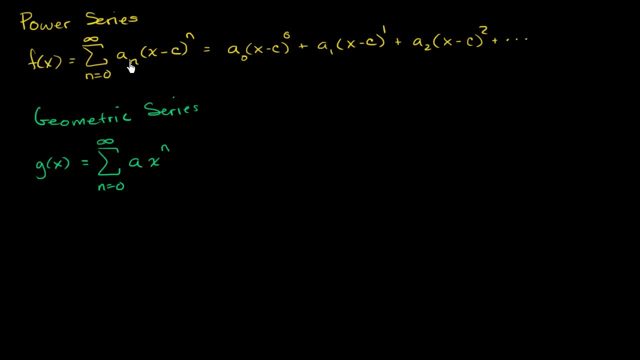 we're going to have the same coefficient a, While over here we have a sub n. we're multiplying by a different thing Every time. up here we're multiplying by the same thing over here, And in this case this particular geometric series. 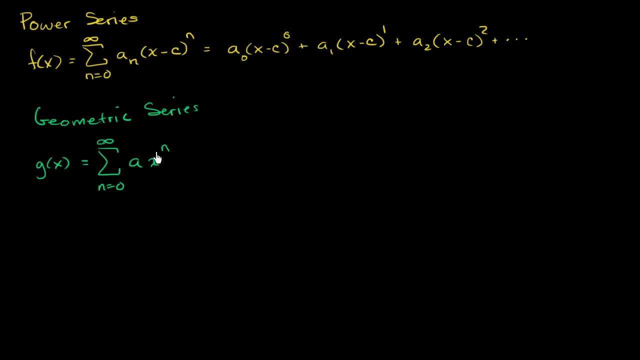 I just made, instead of having x minus c to the n, we have just x to the n. So you could say: well, this is a special case when c is equal to 0. And we can expand it out. This is a times x to the 0, which is just going to be a. 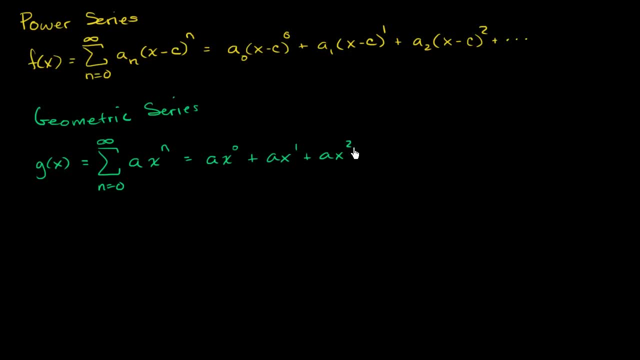 plus a times x to the first, plus a times x squared, And we just go on and on and on forever. Now what's exciting about this is we know that, under certain conditions, this will actually give us a finite value. This will actually converge. 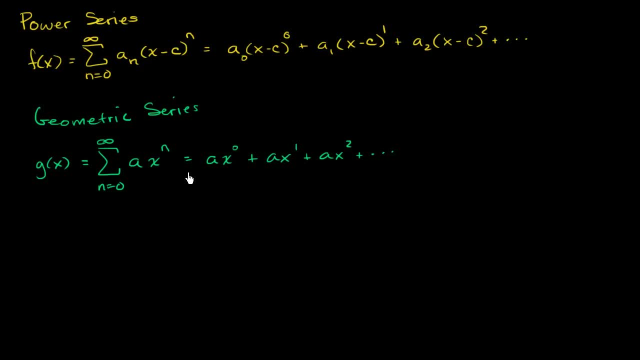 This will actually, I guess, give us a sensical answer. So under what conditions does that happen? Well, this converges as if each of these terms gets smaller and smaller and smaller, And each of these terms gets smaller and smaller and smaller. 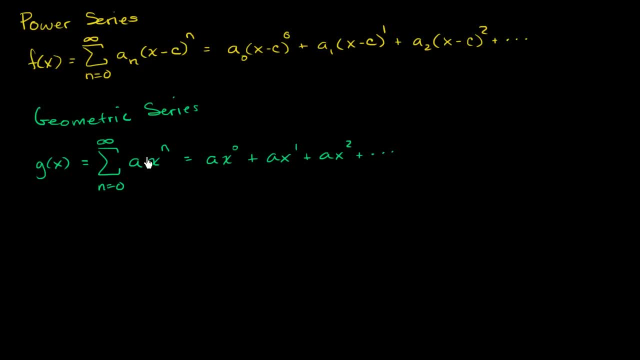 if the absolute value of our common ratio is less than 1.. So let me write that down. So this converges if the absolute value of our common ratio is less than 1.. Or another way of thinking about it- this is another way of saying- is that x is in the interval. 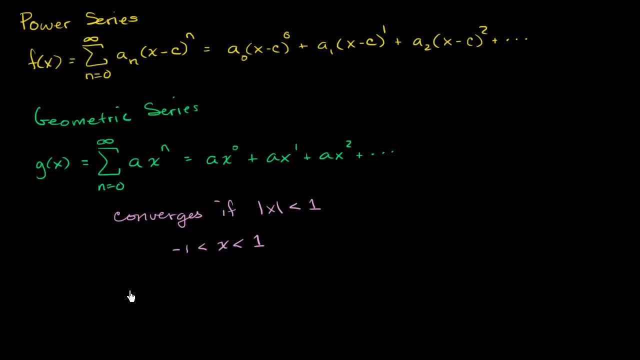 between It's less than 1, and it is greater than negative 1.. And this term right over here now. x is a variable. x can vary between those values. We're going to find a function in terms of x. We call this the interval of convergence. 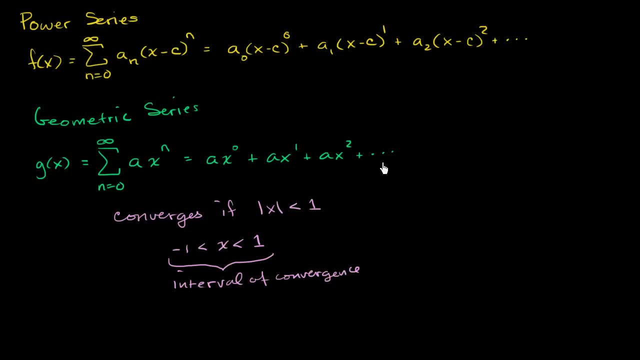 And so we know that if x is in this interval, this is going to give us a finite sum, And we know what that finite sum is It's going to be equal to: If it converges, this is going to be equal to our first term, which is just a. 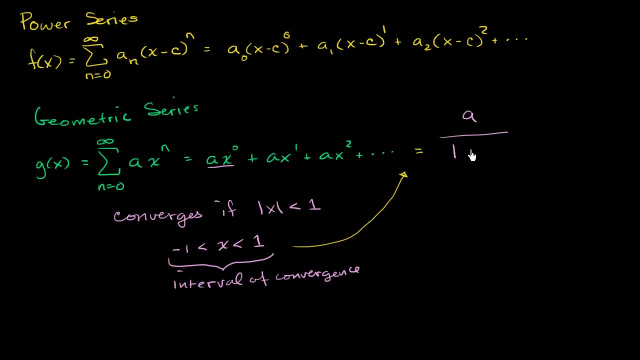 This simplifies to a right over here, Over 1 minus our common ratio. What's our common ratio? Well, our common ratio in this example is x. Going from one term to the next, we're just multiplying by x. We're just multiplying by x right over there. 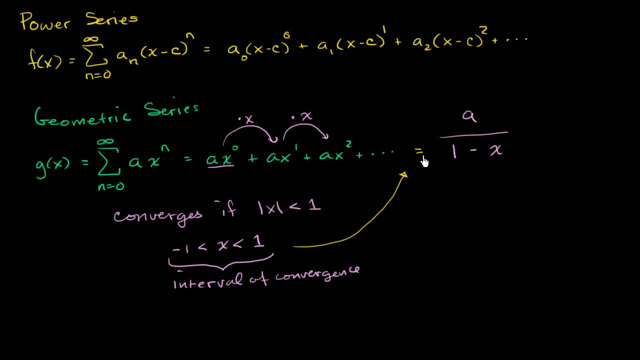 Now, this is pretty neat because we're going to be able to use this fact to put more traditionally defined functions into this form and then try to expand them out using a geometric series. And this whole idea of using power series or, in this special case, geometric series. 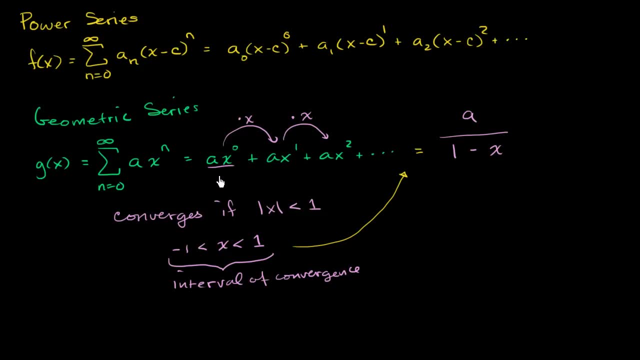 to represent functions has all sorts of applications in engineering and finance. Using a finite number of terms of these series, you can kind of approximate the functions in a way that's simpler for the human brain to understand or maybe a simpler way to manipulate in some way. 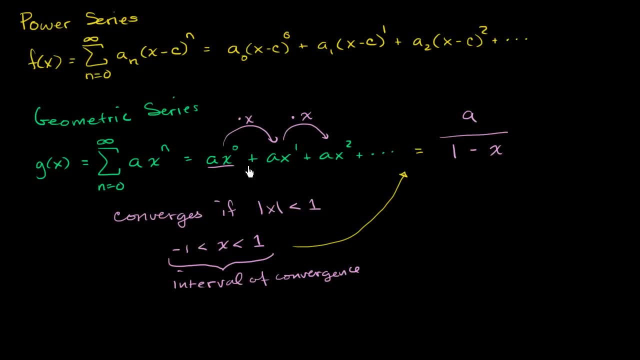 But what's interesting here is, instead of just going from the sum to, instead of going from this expanded out version to this kind of finite value, we're now going to start being able to take something in this form and expand it out into a geometric series. 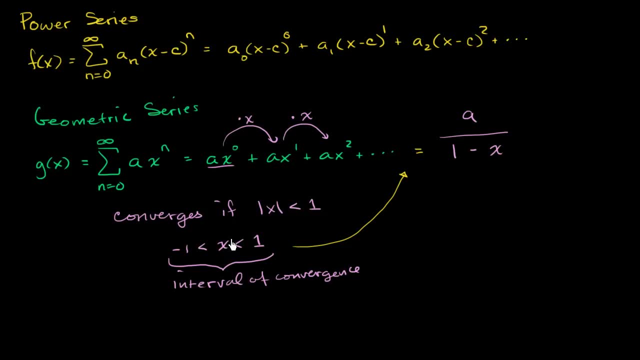 But we have to be careful to make sure that we're only doing it over the interval of convergence. This is only going to be true over the interval of convergence. Now, one other term you might see in your mathematical career is radius of convergence, And this is how far up to what value. 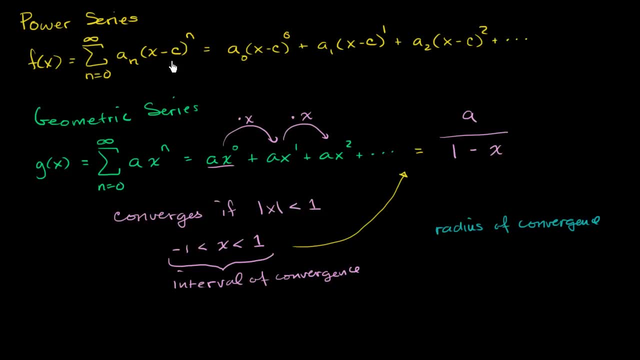 but not including this value. So as long as our x value stays less than a certain amount from our c value, then this thing will converge. Now, in this case, our c value is 0.. So we could ask ourselves a question of: 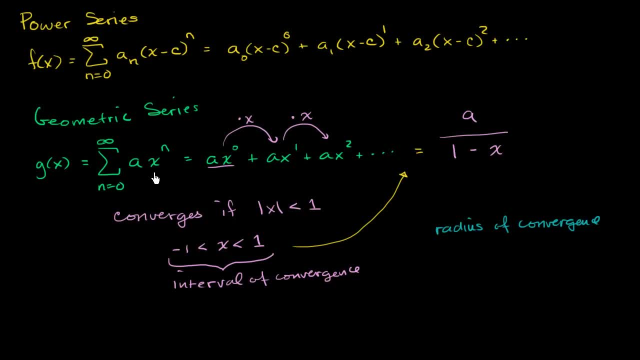 as long as x stays within some value of 0, this thing is going to converge, And you see it right over here. As long as x stays within 1 of 0, so as long as it can get. it can't go all the way to 1,, but as long as it stays less. 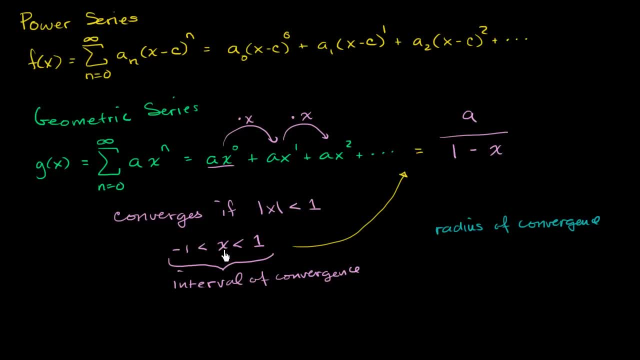 than 1, or as long as it stays greater than negative 1,. so it can stray no more, or I guess it should. it can stray anything less than 1 away from 0, either in the positive direction or the negative direction. 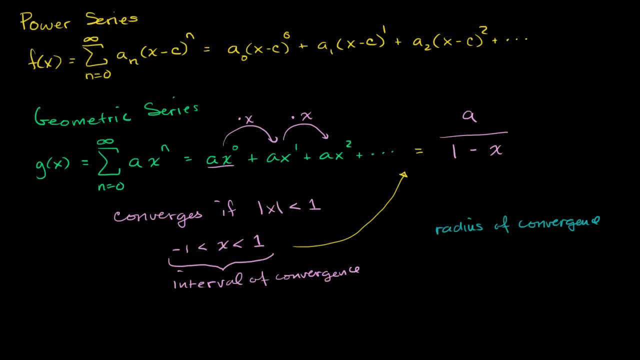 then this thing will still converge. So we could say that our radius of convergence is equal to 1.. Another way to think about it: Our interval of convergence- we're going from negative 1 to 1, not including those two boundaries.